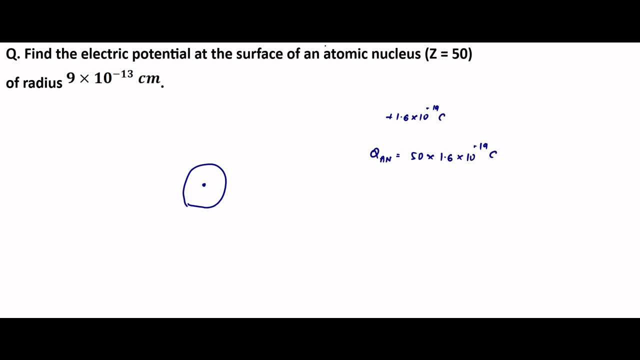 This is the thing Now. we know that we have to calculate this potential at the surface of the nucleus. we have to calculate the potential at the surface. So when we have to calculate it at the surface, we have to consider this radius, the radius of the nucleus, which is equal to 9, into 10, to the power minus 13. 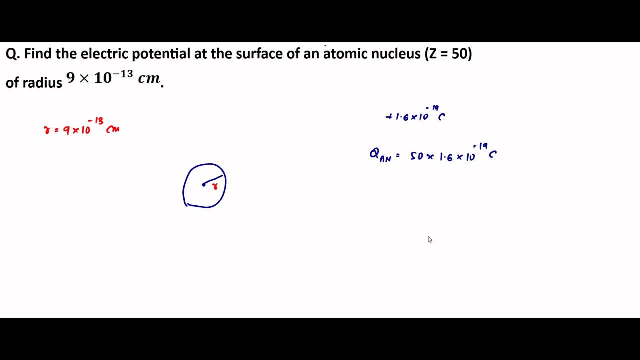 centimeters. Now we know the formula for electric potential at any point due to a charge. So let us say we have a charge here, Q, and we have to find the electric potential at this point, P, due to this charge, which is at a distance of r away from it. So the formula of electric 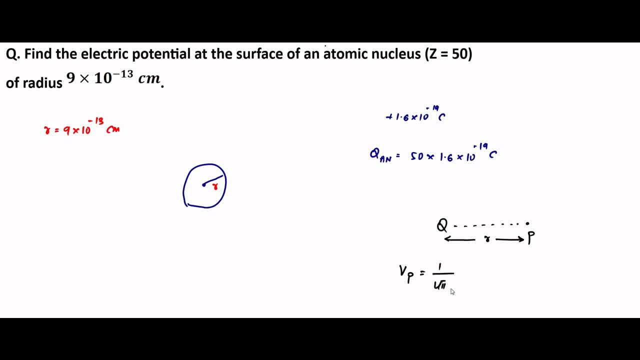 potential at this point P is equal to 9 into 10 to the power minus 13 centimeters. So the potential at the point P is equal to 1 by 4 pi epsilon 0, Q by r. This is the formula. 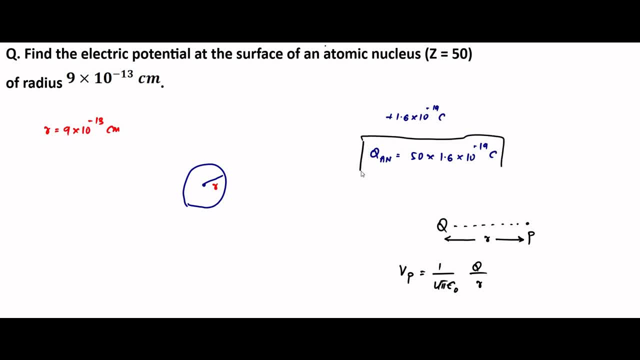 So here we will be doing that Here. the total charge that is equal to this because of the atomic nucleus, positive charge, The potential at the surface, we have to calculate. So we have to consider this as the separation distance r, the radius of the nucleus. So 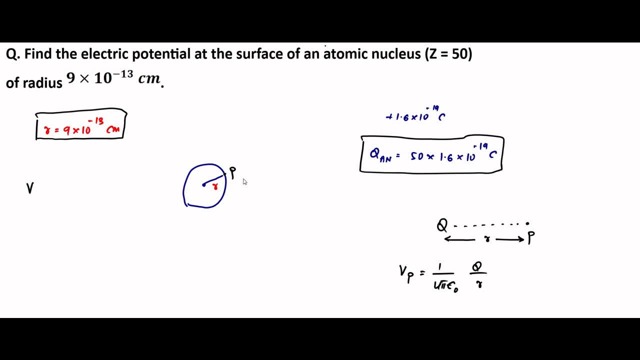 it will be the potential at the surface at this point. that is equal to 1 by 4 pi epsilon 0. total atomic nucleus charge by radius of the nucleus. Let us call it r? n radius of the nucleus. equal to this 1 by 4 pi epsilon 0 part, that is equal to 9 into 10, to the power, minus 13 centimeters. 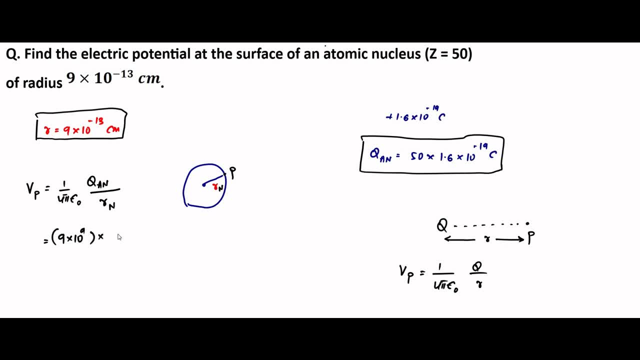 9 into 10 to the power 9.. This total charge, that is equal to 50 into 1.6 into 10 to the power minus 19. coulomb Radius of the nucleus: that is 9 into 10 to the power minus 13 centimeters. So 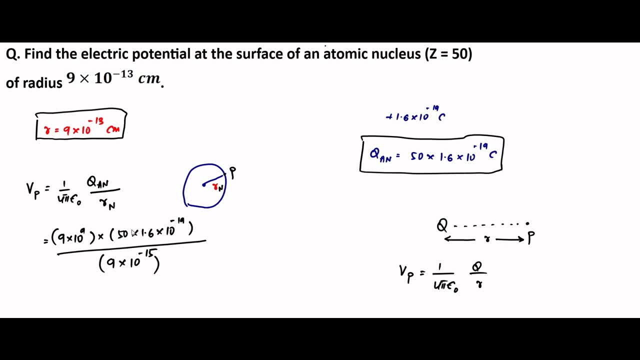 that is 10 to the power minus 15 meters converting into MKS units. So the result that is coming: it is equal to 8 into 10 to the power 6 volt. Okay, That is the result: 8 into 10 to the power 6. 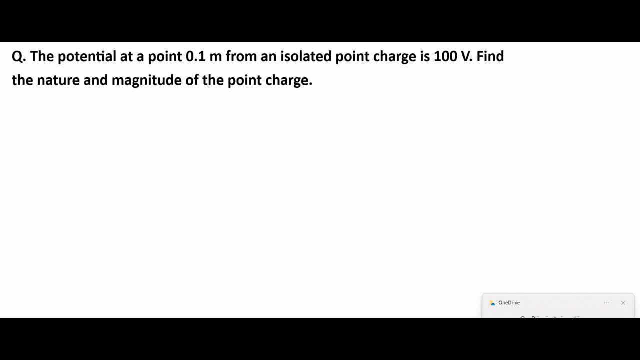 volt. That is the answer. So here is another question on electric potential. So here it is: given that the potential at a point 0.1 meter away from an isolator is equal to 0.1 meter, So the isolated point charge is 100 volt. We have to find the nature and magnitude of the point charge. 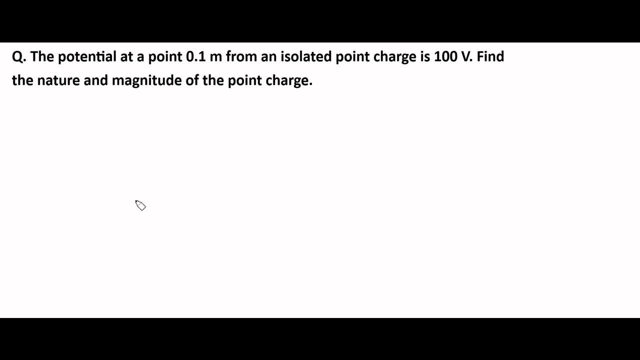 So here the question is: the situation is that we have an isolated point charge, Okay, And at a distance of 0.1 meters from it. So we have to find the nature and magnitude of the point charge. So the electric potential at this point is equal to 100 volt. Let us say this point charge isolated. 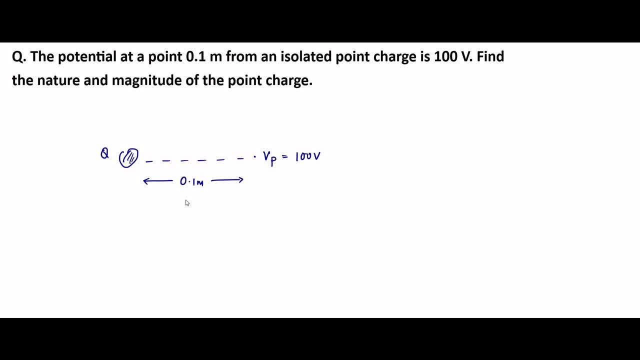 point. charge is Q. Now we know, and this is the distance separation distance R. Now we know, that electric potential at any point is given by 1 by 4 pi epsilon 0.. Epsilon 0 only because nothing has been mentioned whether the charge is placed in any 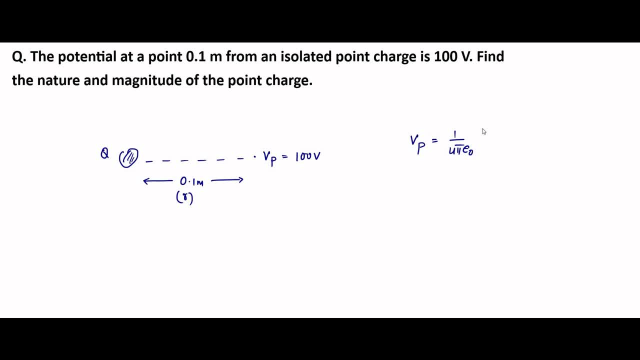 other medium. So we have to assume it is free space or air. So epsilon R relative permittivity is 1.. So that is equal to Q by R, the gap, So here it is given the voltage is 100.. This is 9. 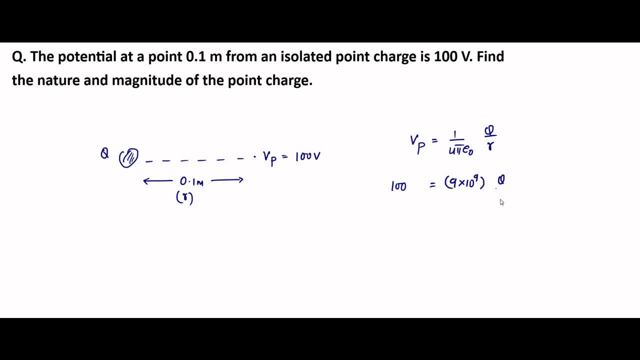 into 10 to the power 9.. Alright, it is a little bit impossible in functionally to prove, So in that case we will only use 0.01 per second, per second at 0. Поэтому R anone transistor of 0 by 4 pi, epsilon 0, Q. 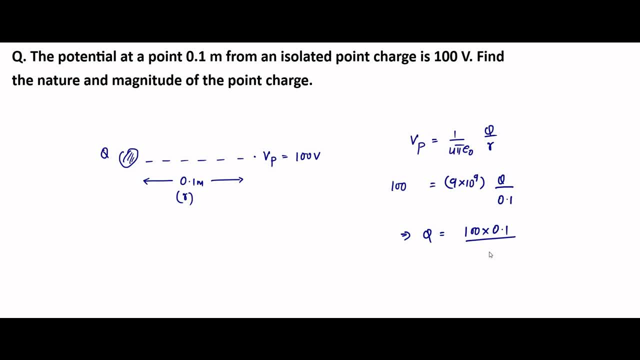 by 0.01, we have to find Q. That implies Q is equal to 100 into 0.1, by 9 into 10 to the power 9.. So it is coming. So it is plus 1 point 1 into 10 to the power minus 9. coulomb. Now this: 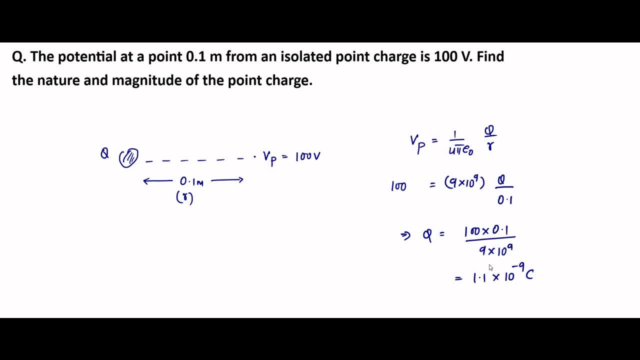 or 1.1 nano. that So very simple and straightforward. this is the solution. So here is another question on electric potential. So here it is given. find the electric field between two metal plates which are separated 3 millimeter apart and connected to a 12 volt. 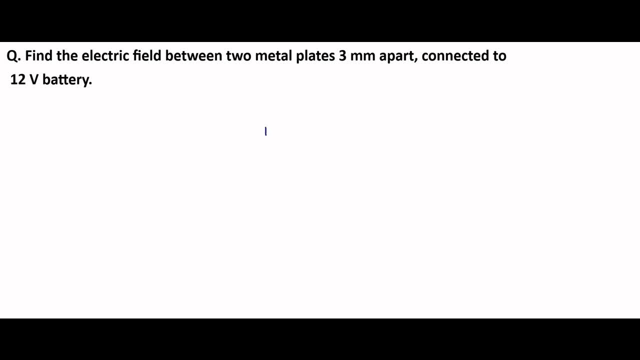 battery. So basically, here we have two metal plates which are connected to a 12 volt battery, And the separation distance is 3 meters. So we have to find the electric field between these two plates, plate 1 and plate 2.. So here 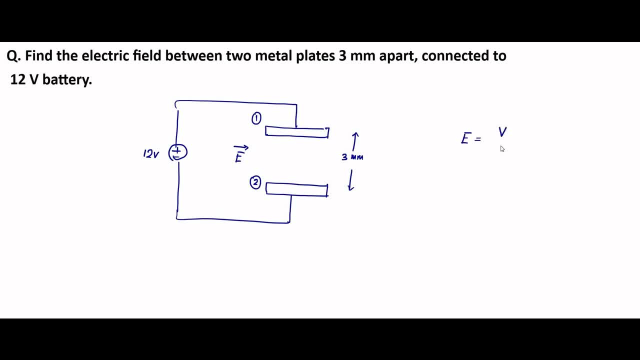 we know that electric field is electric potential or potential difference between two points divided by the separation distance. Ok, And here that is why, when we use the unit of electric field, we use Newton per coulomb or volt per meter. these two units can be used to represent electric field. 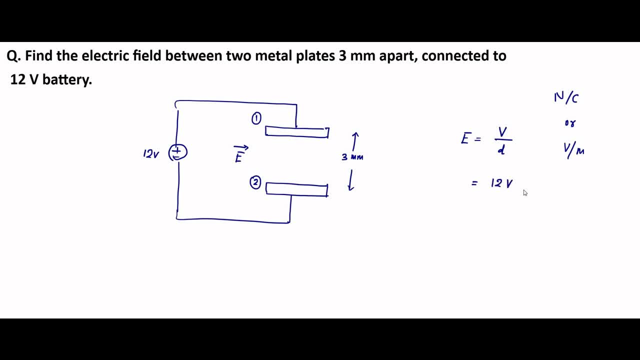 So here the potential difference is 12 volt and the separation gap is 3 millimeters, which is 3 into 10 to the power minus 12 volt, 1.6 meter. and here it is given we have a separate joint chain at volume and there is theとか delta meter and the other part of a haciendo unit, 14.5 with 6 and 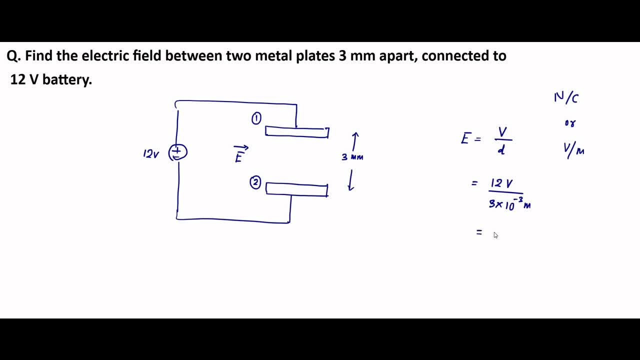 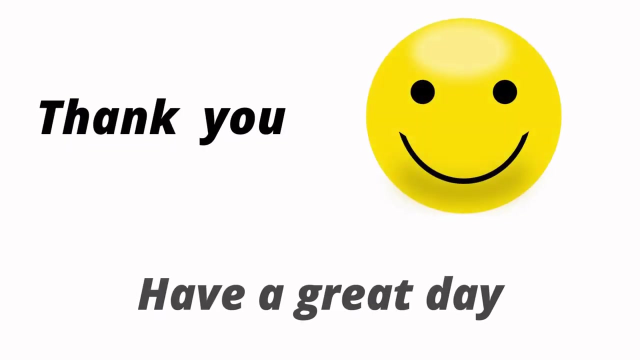 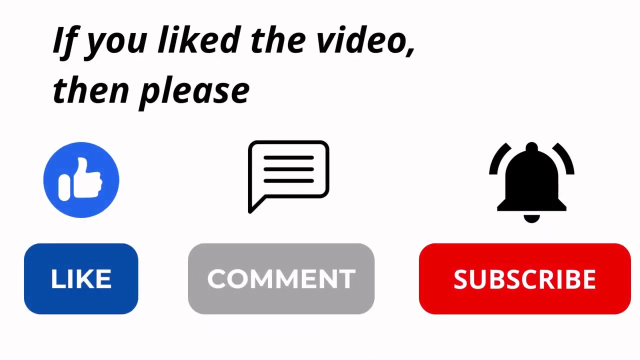 3 meters in MKS units, So it is 4 into 10 to the power 3 volt per meters. That is the electric field between plates 1 and 2 here. So very simple and straightforward you.